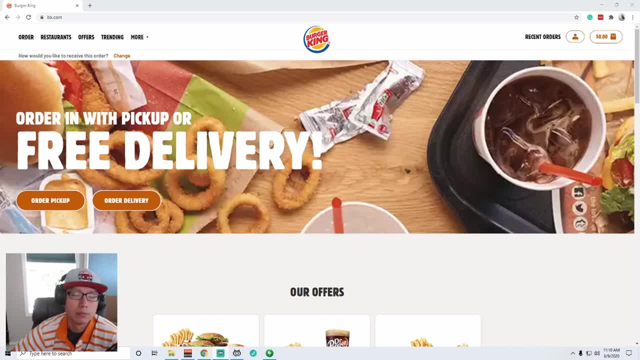 I was missing one Whopper, I did what any reasonable person would do. First thing I did was to call back the driver. The driver didn't answer the first time. I called him back again. He answered, but then he pretended like he couldn't hear what I was saying. I then texted him. 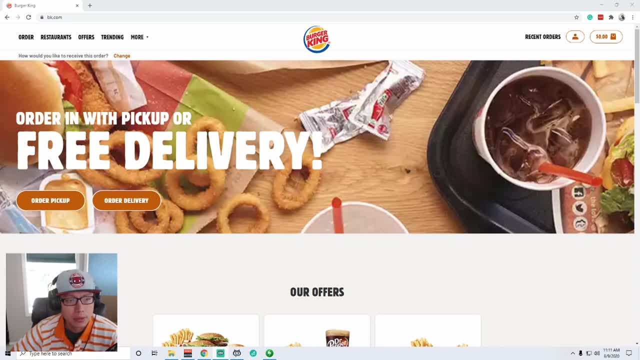 but no response To this day. no response. So the driver was working for DoorDash. So Burger King uses DoorDash as their delivery system when you order from their website. So I went on to customer service on DoorDash and they're like: sorry, dude, we can't do anything for you because you didn't. 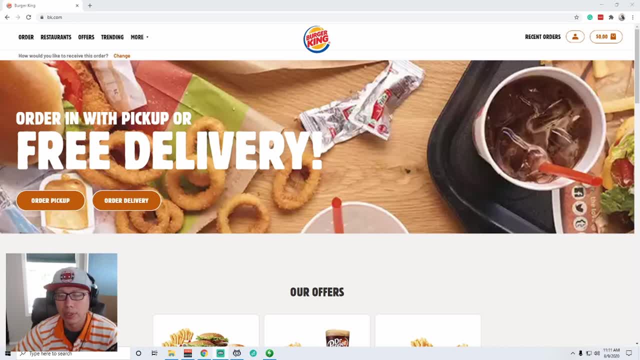 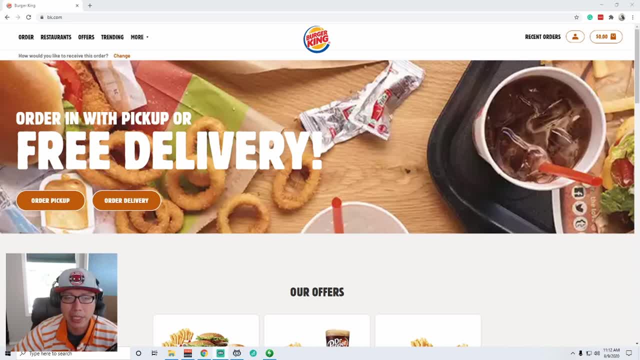 And pick up a single Whopper when I had ordered for a delivered Whopper. So long story short. this is kind of why I want to test the Burger King app, But also other things. that I found was while trying to make my order, the website wasn't working properly when I was trying to do certain. 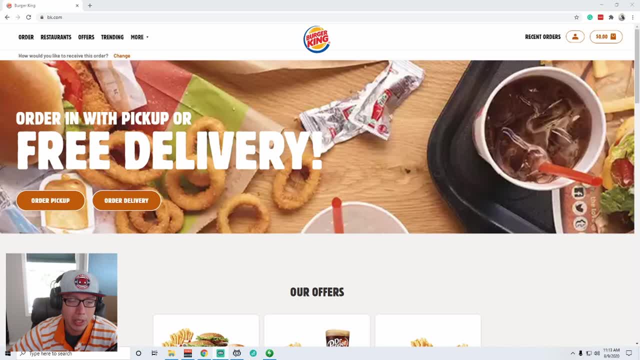 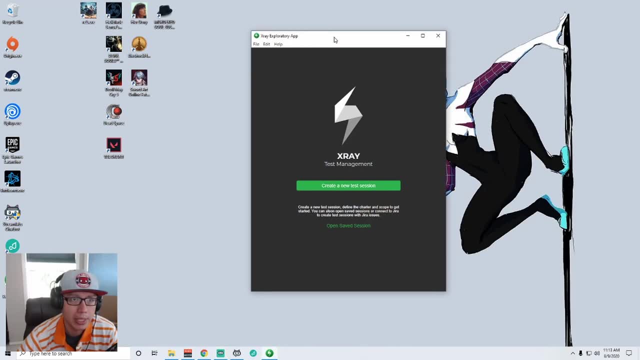 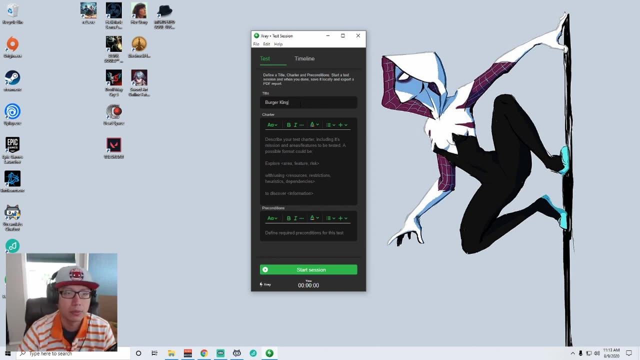 things, And I will point those out today as I run across them again. But let's go ahead and start this up. So first things first. I'm going to use this X-Ray Exploratory app. So let's a new session here and we're going to call this burger king and let's see charter, let's see. 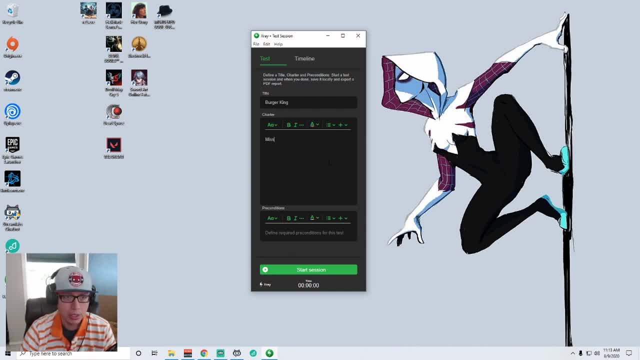 describe your test charter, including its mission. so mission, mission, uh, order, food objectives- have it your way. so that's, that's burger king's slogan. right, have it your way. or at least it used to be. maybe i'm really old, all right, so good enough, we'll figure things out. 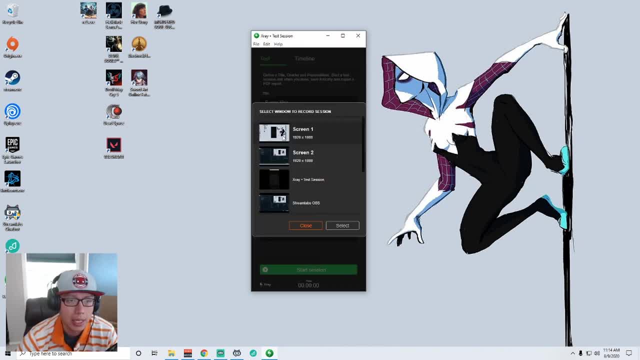 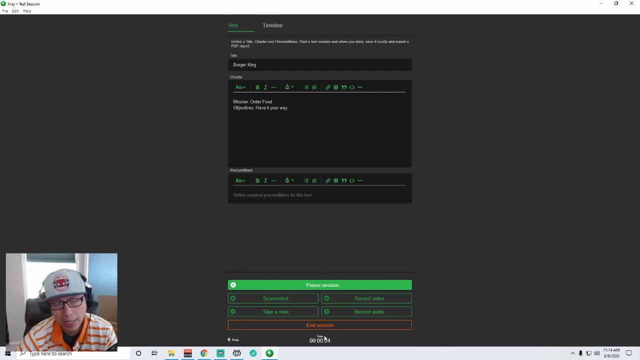 on the way, this doesn't really matter, so let's go ahead and start the session and let's see. i want this screen, sure, okay, so timer started. i'm going to spend about an hour my time looking for stuff, but i'm i'm just going to cut the video to bits and pieces that are important to you guys first. 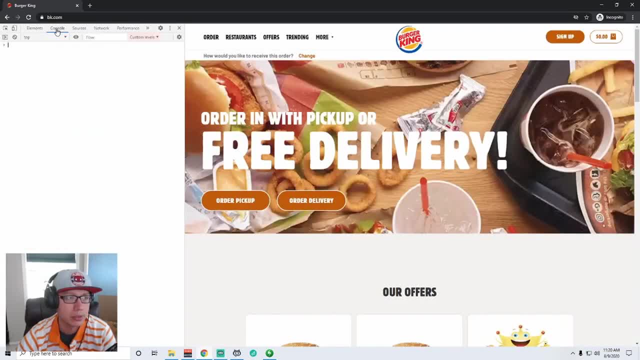 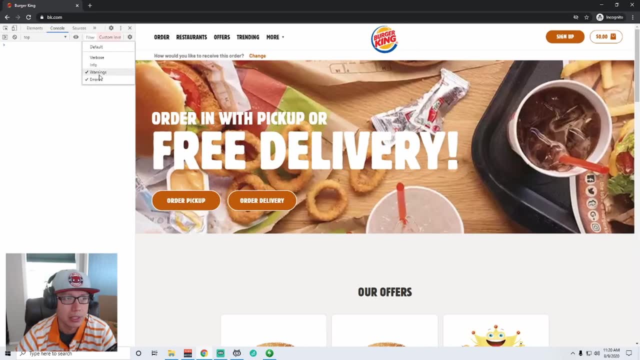 thing i'm going to do on the website is i'm going to hit inspect and go to console just so that i can see if there's any errors popping up when i'm doing things. so, uh, i have my level set to just show warning and errors. so if 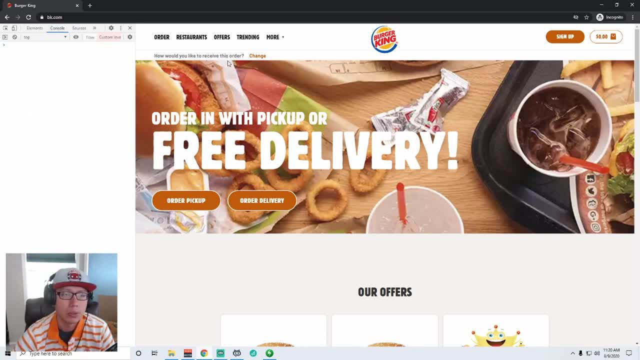 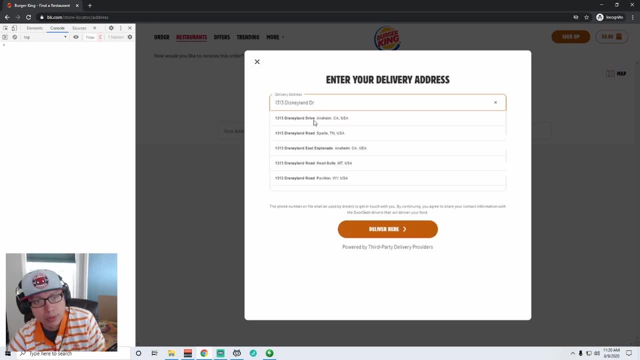 you. if there's any warnings or errors, then it should show up in there, all right? so what i'm going to do is order delivery, because that's what i did. um, i have disneyland's address in my clipboard, so let's do that, and we want the one in anaheim, california. and then let's try a fake phone number. 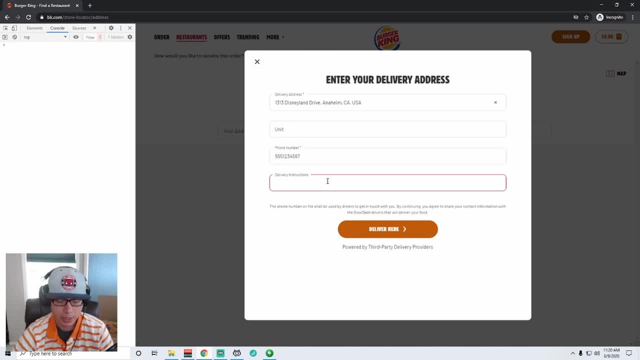 okay, and let's see delivery instructions. don't forget my food. all right. so it looks like it knows that this is not a valid phone number, so i think it's probably hinting off of the area code. so i can do like a 206 and let's try that. so that doesn't work either. so it has something in it that is. 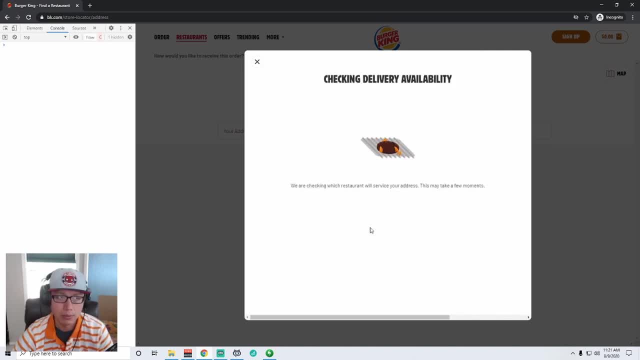 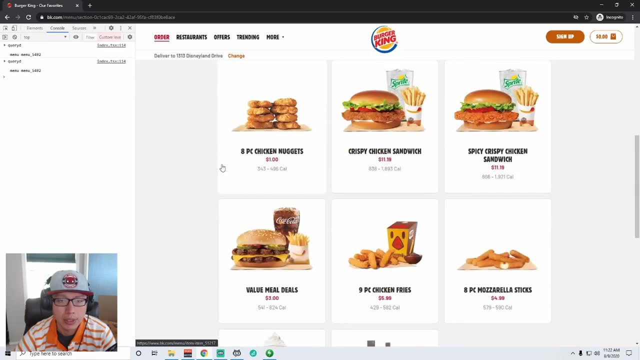 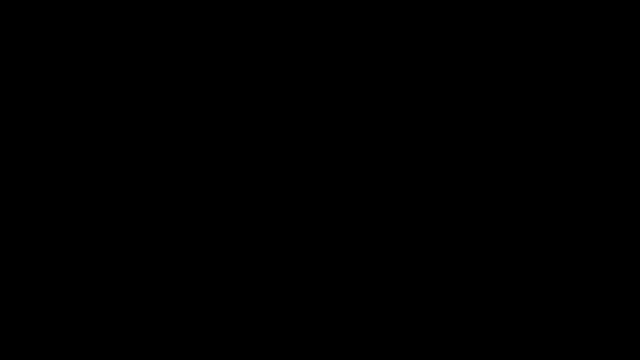 telling it it's not a valid phone number, but that one apparently is. so that's cool. let's go to our favorite and let's see if we can find anything. i'm i'm looking for for some deals. it doesn't look like you got any deals. 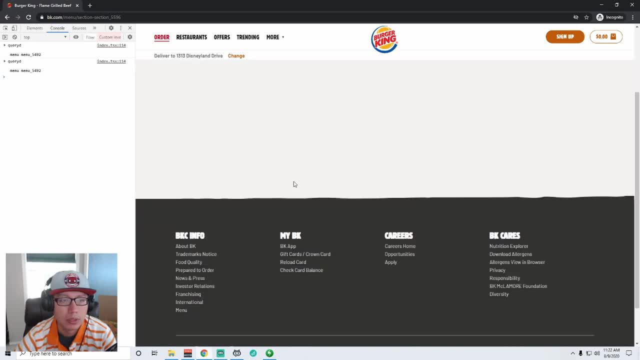 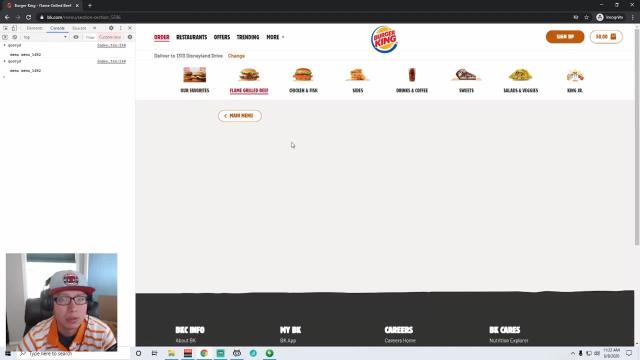 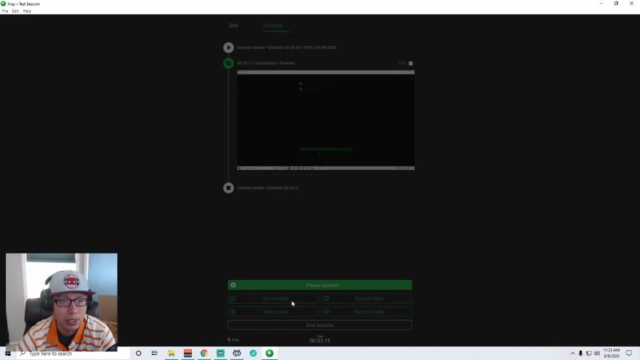 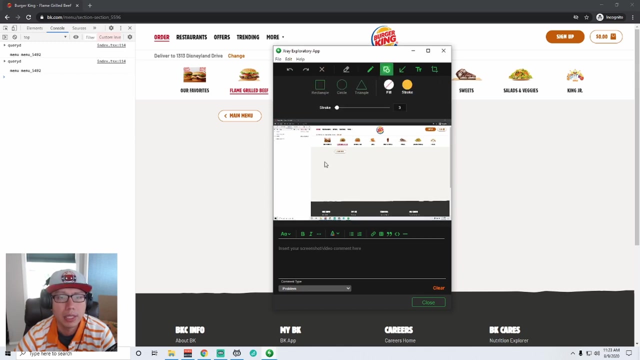 oh fun, you see that. so if i go to flame grilled beef, i get a. i get a blank page here. so that's let's, let's take a picture of that. so screenshot. so there's a screenshot. um, you can see that there's no, there's no things here, there's no flame grilled beef. so if i click 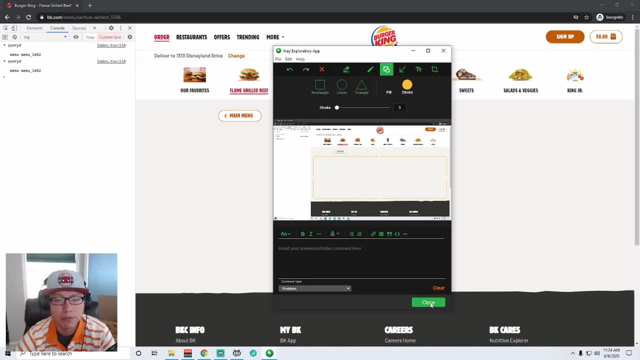 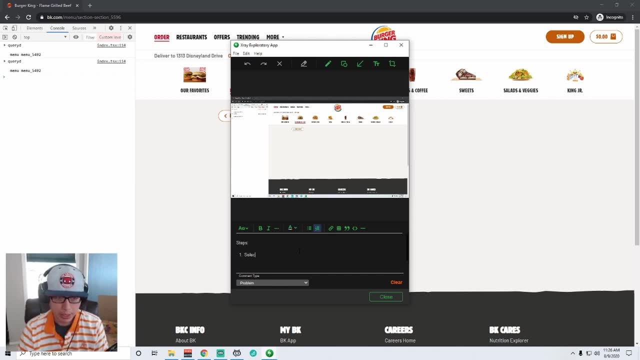 on that section. there's no stuff there, right, and put some steps in. so steps one: select- i'm just gonna not put the one there, i'm just gonna say select delivery order. and then second thing is: select flame grilled beef, and then actual, i'm going to say nothing is displayed, okay. 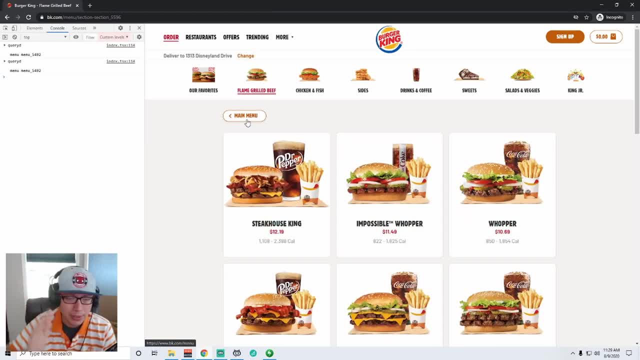 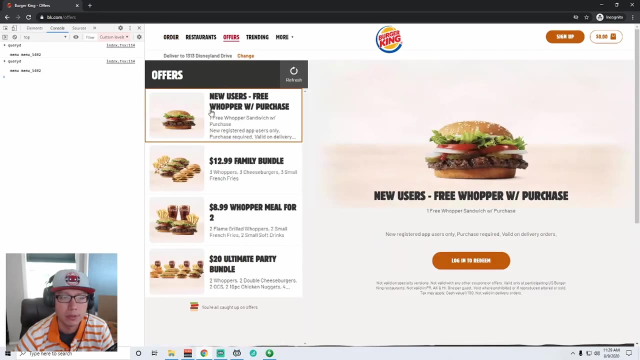 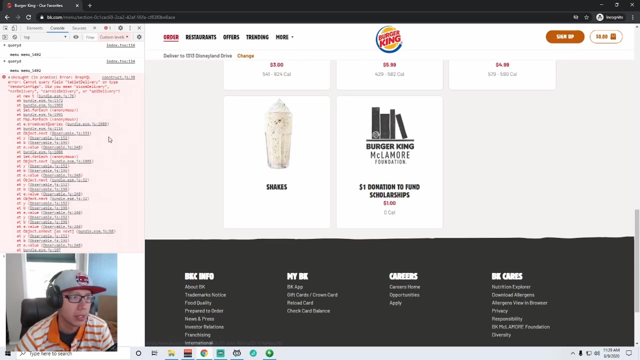 all right. so this, this is the fun part. so i had something bad happen, so i, i cre i found a bug, but now i need to figure out exactly what i did to make that bug happen. so let's see um offers our favorites. i remember looking at this: oh there we go. so, uh, graphql error. so uncaught error. graphql. 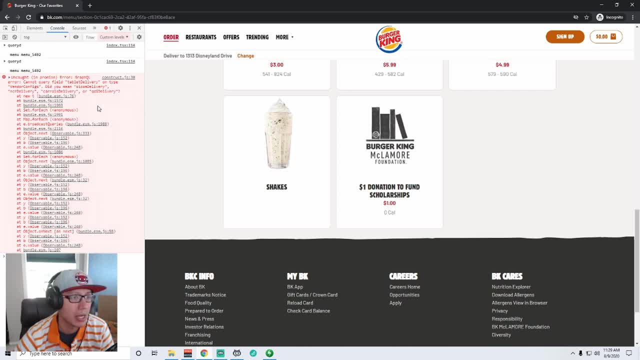 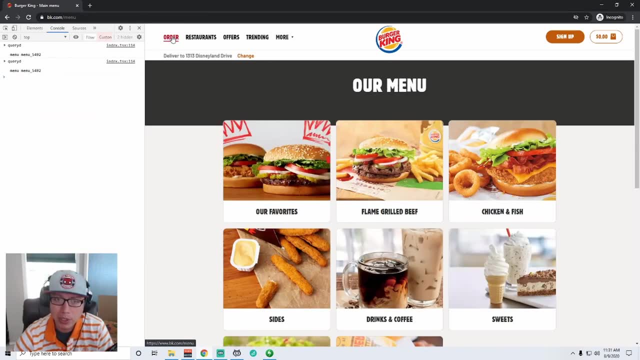 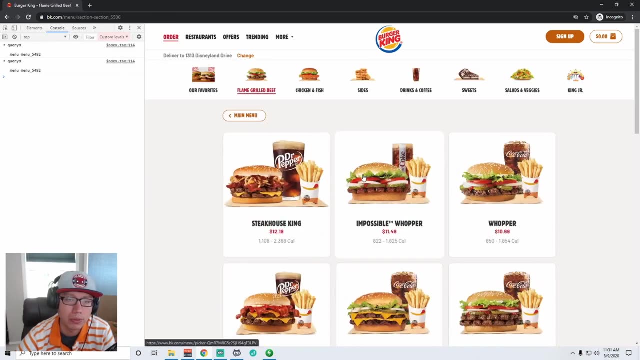 error cannot query field tablet delivery on type vendor configs. did you mean psycom delivery? so i'm not sure what i did to make that happen. a big part of uh exploratory testing is that you just explore, just click around, see things. there's no structure, there's no rhyme or reason behind things. you're just kind of trying. 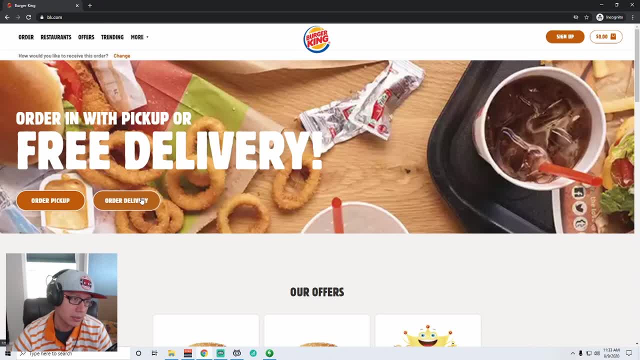 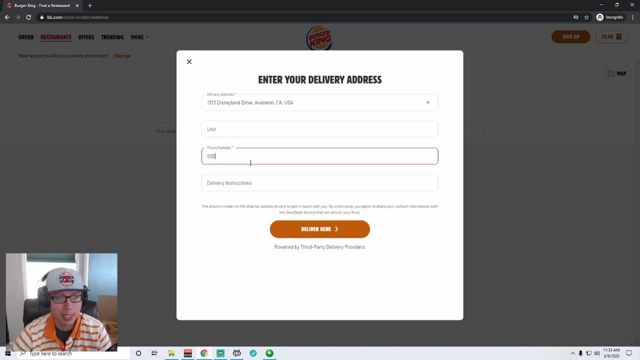 to do things in a user sort of way, okay, so let's, let's take our time. so let's, let's remember what we did before. so before we did this, um, we actually had a bad phone number right, and the fact that they let me do this at all is ridiculous. that that's come on, guys, all right. 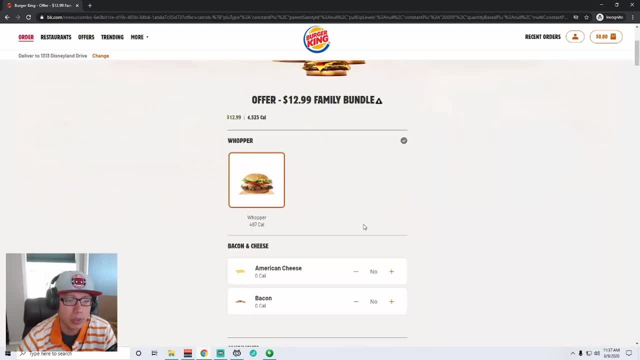 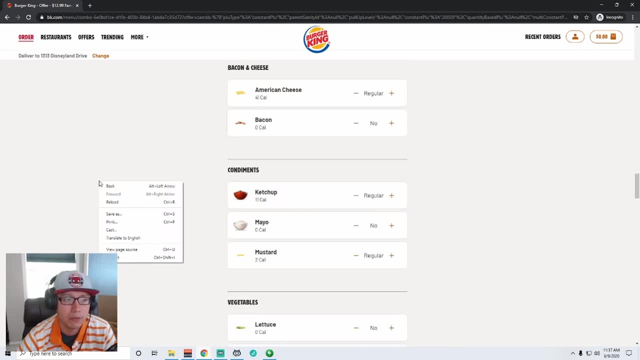 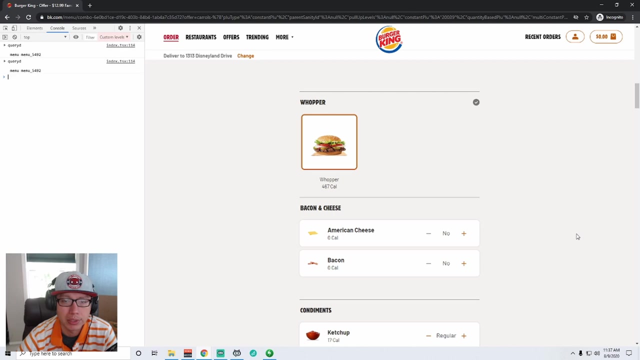 let's try this, okay, so add to mobile order and let's let's do one so you can do all this customization stuff here. that's all fun and games. so typically what i would do here is i would mess with all these things at, go do plus and minus and plus and minus and c, make sure everything works. 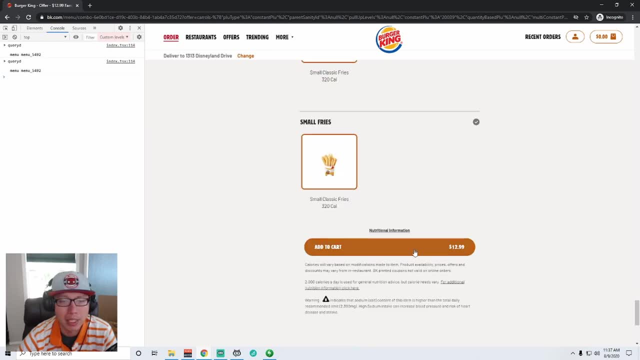 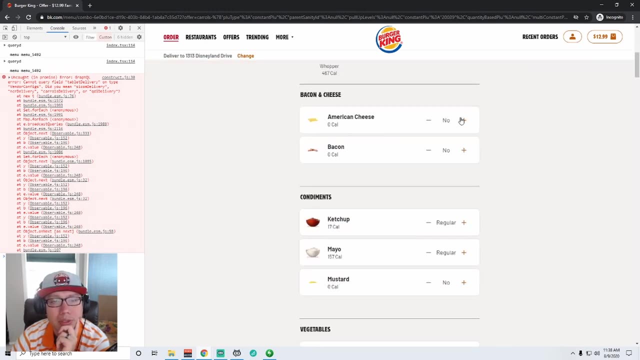 right now. let's just take the default, so this is called happy path. take the default, so let's add another one. but this time i'm going to add a new one. so i'm going to add a new one because i'm going to mess with stuff. so it says no cheese, that's. 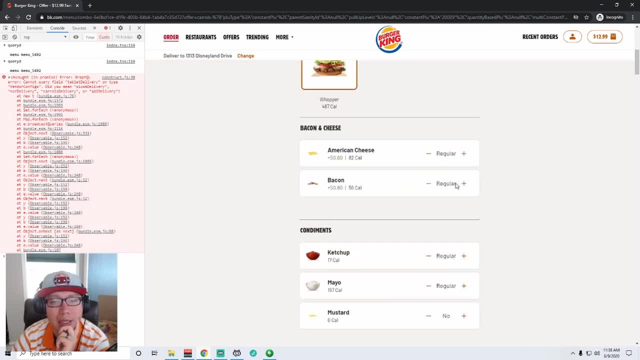 going to add regular cheese. you can't add extra bacon. so this first guy here: i'm going to add extra. i'm just going to hit the plus sign once on everything. so whatever it was as the default, it's now plus one. okay, the second guy: actually, let's go ahead and just submit that. let's just 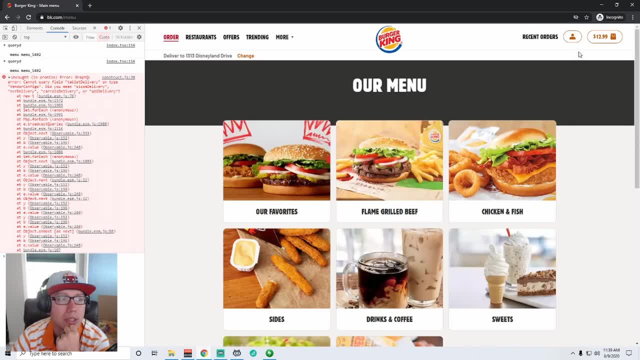 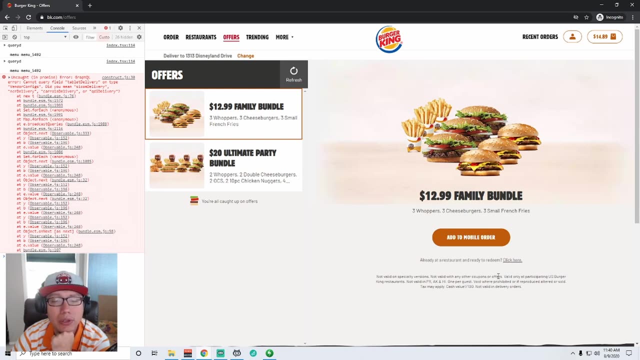 make sure that works before i, because it's going to get complicated if i don't say anything. what's happening here? we go to add to order, so it says add to order, but what happened? do you notice that my cart did not increase? not valid on specialty versions. not valid with any. 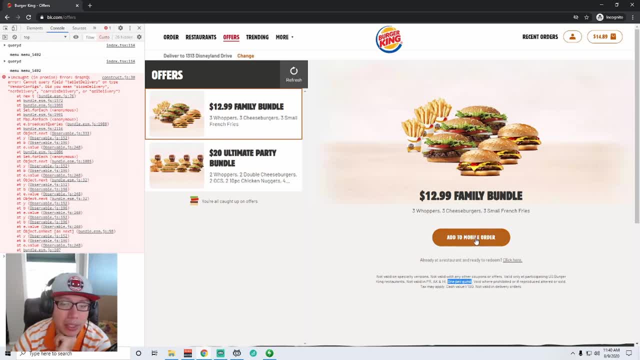 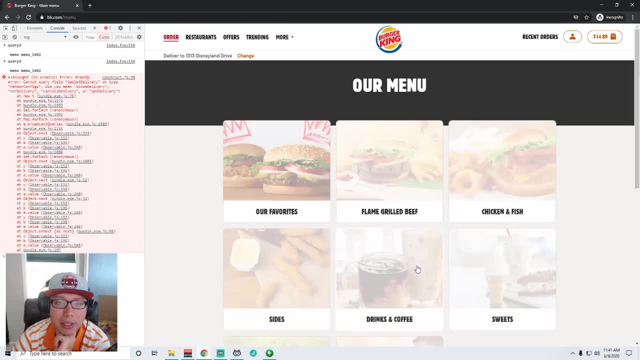 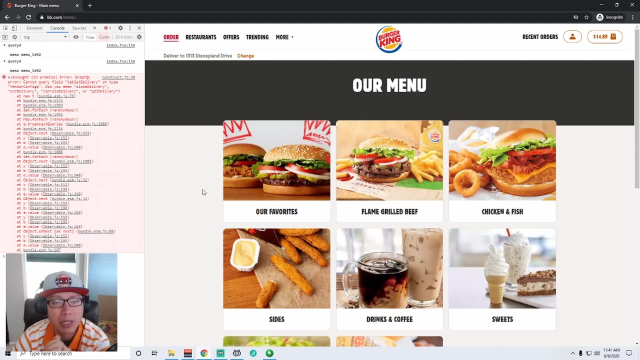 other coupons or offers valid only at participating us burger king restaurants. not valid one per guest. so one per guest is the thing. the problem here is that i have one in my cart. i do all my stuff, i hit add to cart, tell me that it didn't add it to my cart, it just silently fails. so that's, that's no bueno, if there's. 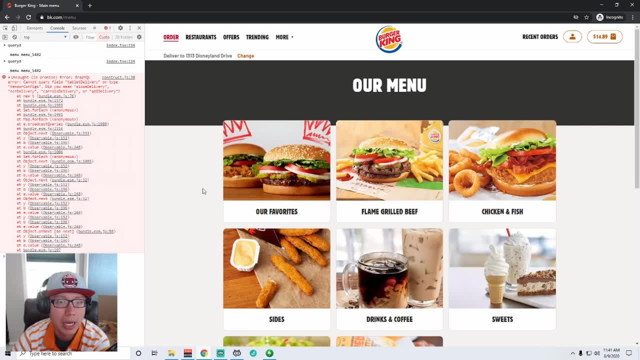 no error telling me that i have a problem. then i'm just going to try again and i'm going to try again and it's just going to make me mad and i don't know why it doesn't work, because me, like most other people, when we're ordering food or using websites and stuff, we're not reading the fine. 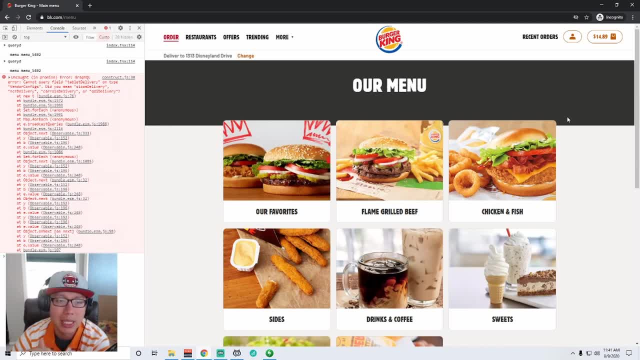 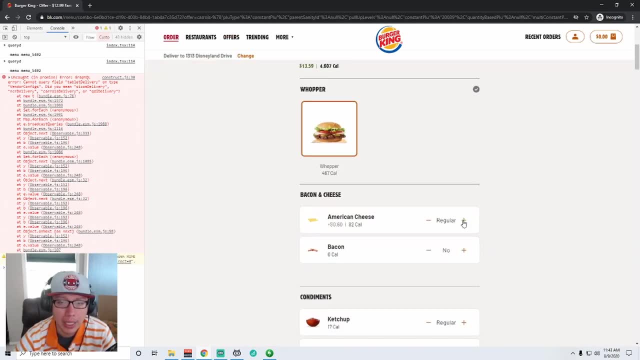 print that says one per order. you need to let us know when things are not working. you can't just snope out of it. let's try one more. so i'm gonna add- i'm gonna load this guy up, so i'm gonna click the plus sign everywhere. you're gonna get extra everything, whether you like it or not. 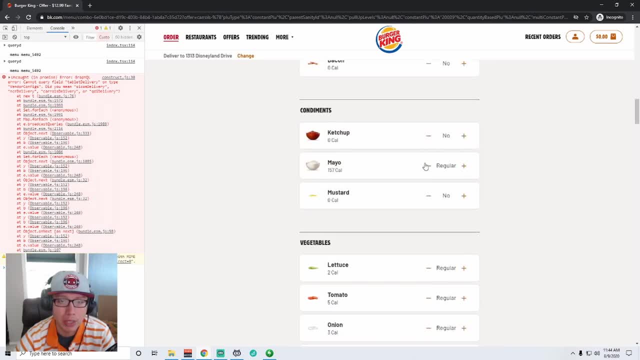 and then this one. i'm gonna snope out of everything. so basically, somebody wants the whole buffet and then somebody just wants some meat and toast. add to cart. that works, check out, let's just make sure. all right. so here we go. we're seeing all these errors here, just for fun. 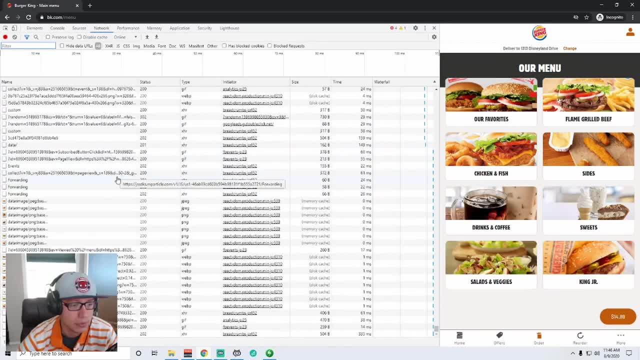 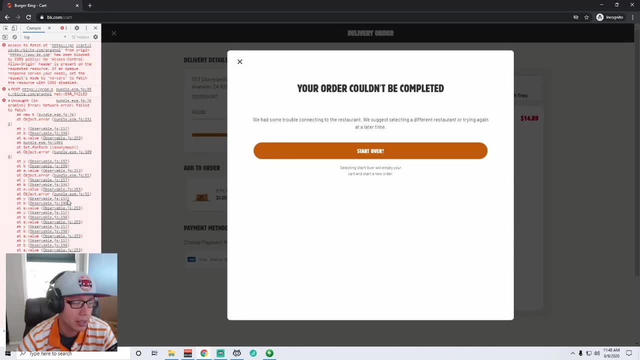 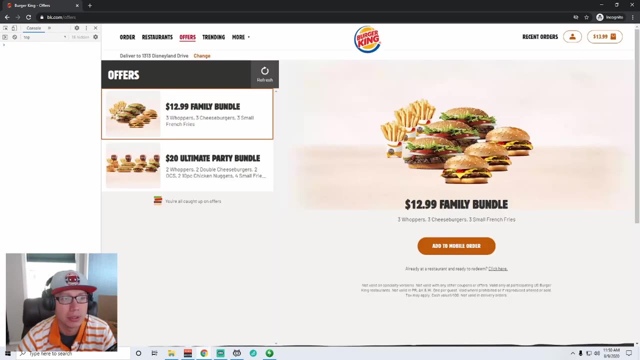 let's, let's go a little deeper here. let's go to network. let's see if we have any errors. graphql failed, so you cannot add and subtract items from two different burgers at the same time. why is there a refresh button here? i just noticed that. that is really silly. 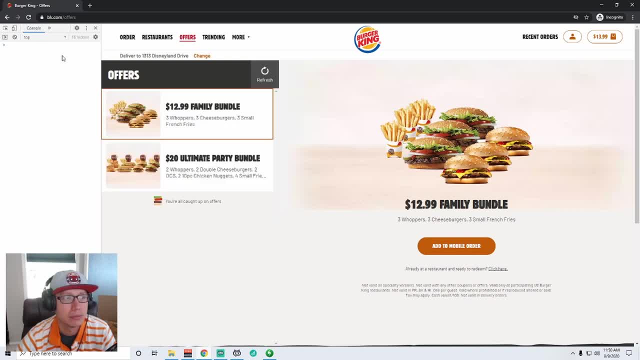 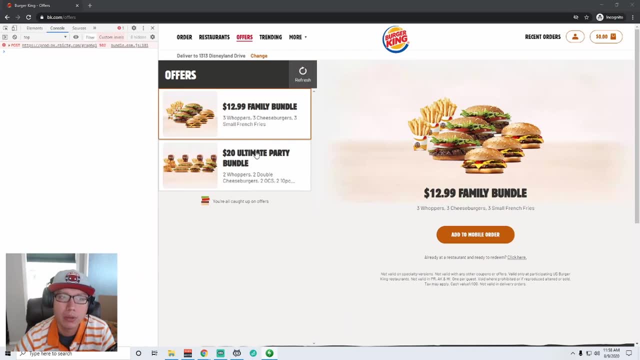 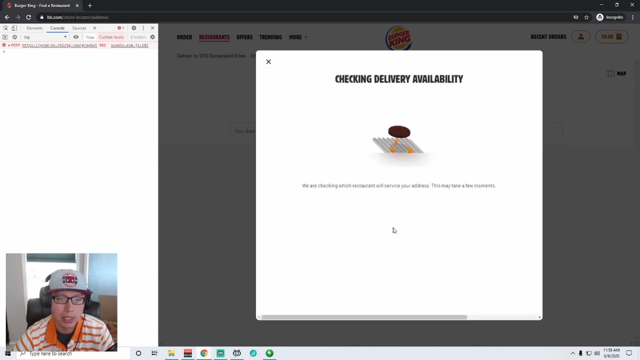 okay, so this, this, this one up here that the browser gives us is not good enough, so you have to have your own customized refresh button. so i really don't like that. when you choose a delivery, you put an address in like this, you select it and hit say deliver here. 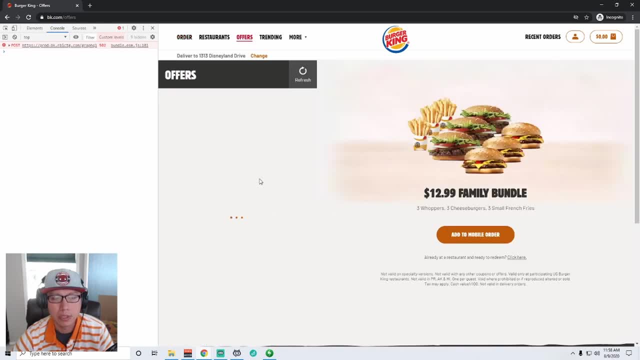 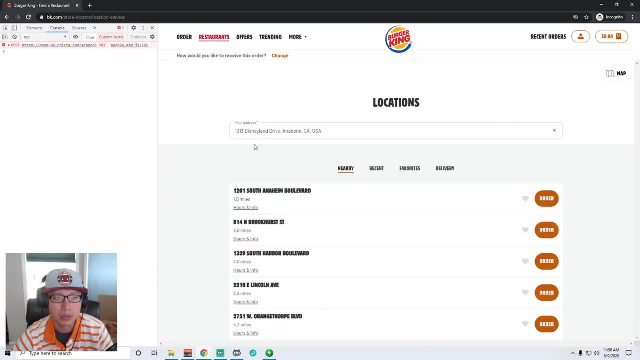 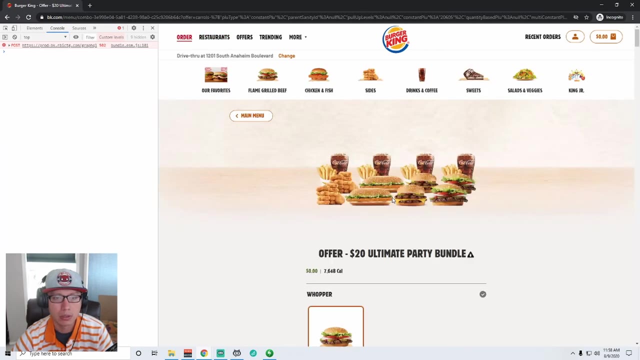 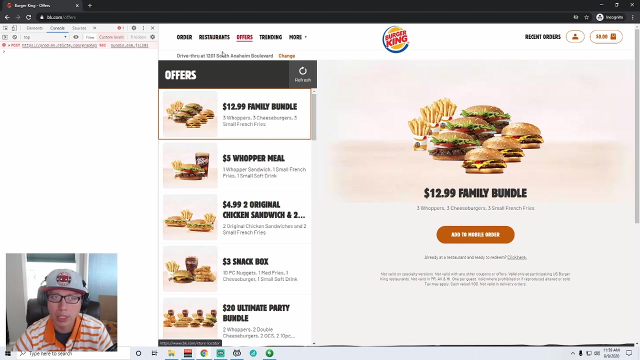 and then you go to offers. you only get those two offers. but if you go to here, actually if you go to restaurants, put in your address, do this and then select the specific restaurant and you go to offers, then you get all of this. One doesn't give you all this stuff and the other does, So it should be the same workflow. So that's. 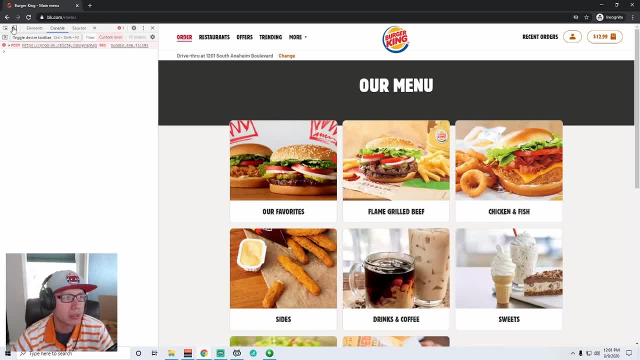 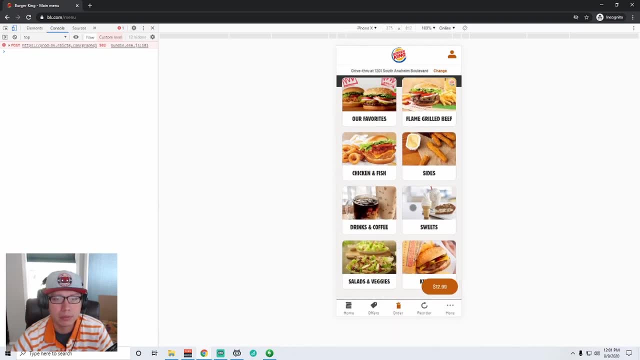 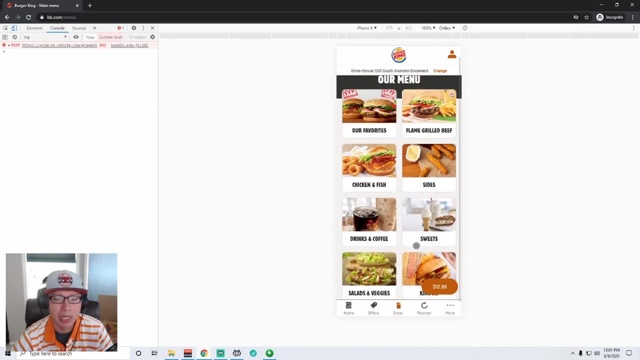 definitely an issue here. Let me play around with the responsiveness a little bit. So here we go. So we are in. let's do like an iPhone X, Cool. So this is not good because the button is overlapping the thing, So you can't actually see what it is. Okay, I'm confused. The buttons are 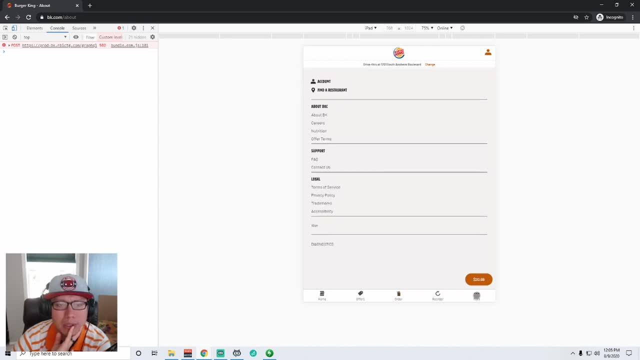 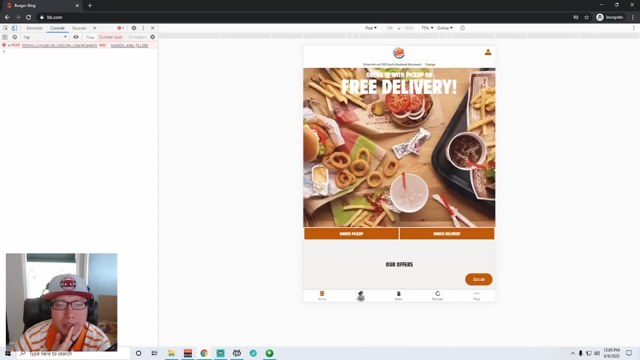 different. What's more, do More is the menu. Okay, How do you close the menu? You can't close the menu, Oh my goodness. All right, I think I'm going to stop here. This kind of shows that even a 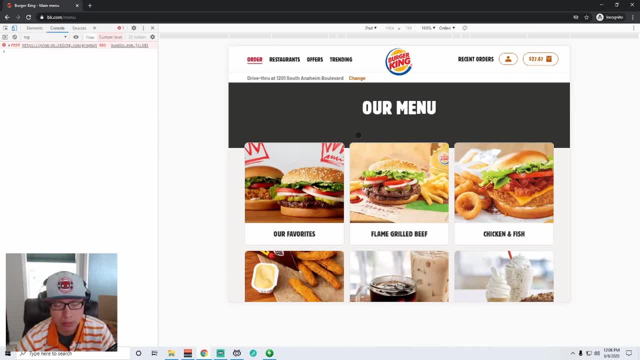 corporate, multi-billion dollar company that has tons of money and resources at their disposal can have websites that are semi-functional and that they have issues. So this really shows you the importance of QA in a IT department. You can't just have developers, You need somebody. 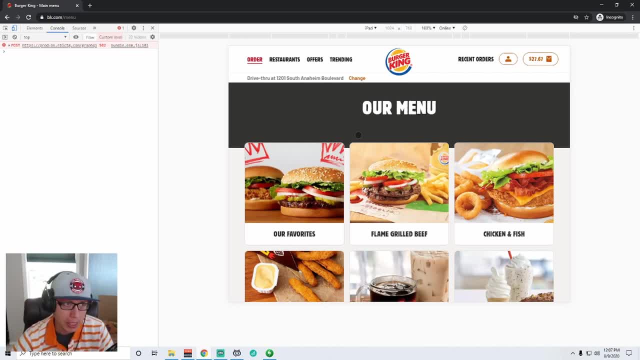 to QA the stuff and make sure that things are working the way they are. For me, customer experience is always the thing. So the other week I spent probably like an hour trying to order the darn Burger King that I still never got my Whopper. So last week I spent probably an hour trying to order that $12.99 meal with modifications.